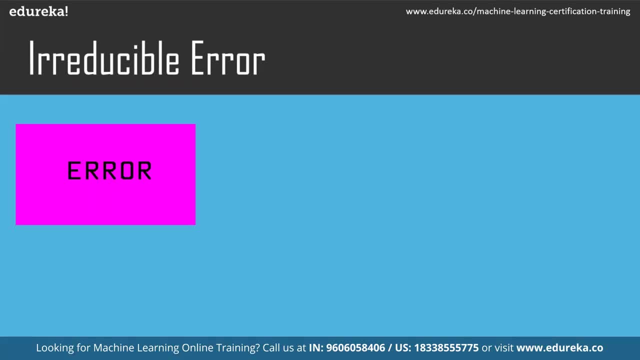 in machine learning is assessed based on the prediction error, on a new independent, unseen data set. Now, error is nothing but the difference between the actual output and the predicted output. to calculate the error, We do the summation of the reducible and irreducible error also. 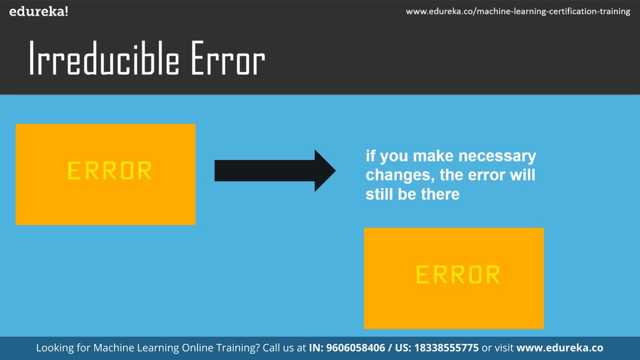 known as bias variance decomposition. Now, coming on to irreversible error, It is nothing but those errors that cannot be reduced, irrespective of any algorithm that you use in that model. It is caused by unusual variables that have a direct influence on the output variable. So, in order to make your model efficient, we are left with the reducible error that we 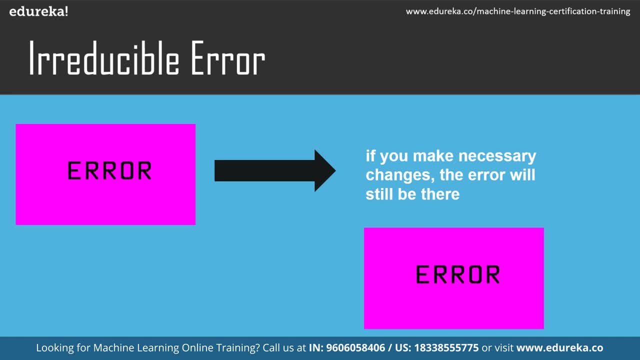 need to optimize at all costs. Now, reducible error has two components, that is, bias and variance. Presence of bias and variance influence the model's accuracy in several ways, like overfitting, under fitting, Etc. and let us take a look at the bias and variance to understand how. 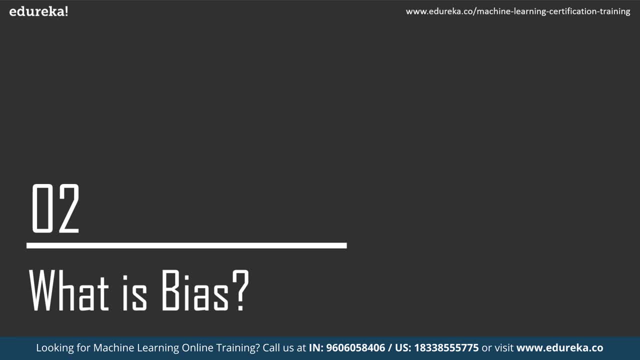 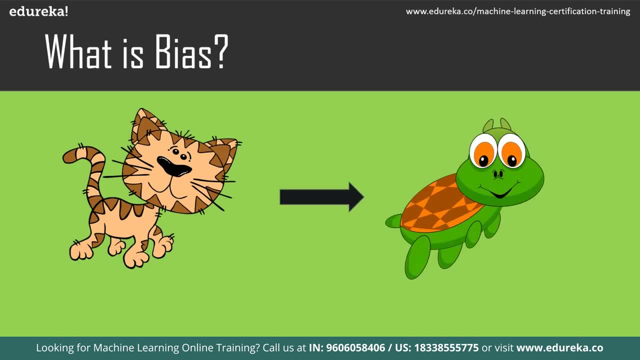 to deal with reducible error in machine learning. So let's understand what is bias in machine learning. bias is basically how far we have predicted the value value from the actual value. We say the bias is too high if the average predictions are far off from the actual value. 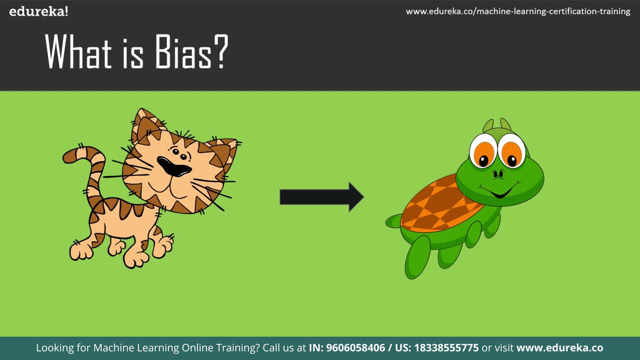 So in this case the bias is clearly very high, And high bias will cause the algorithm to miss a dominant pattern or relationship between the input and output variables. And when the bias is too high, it is assumed that the model is quite simple and does not feed them the complexity of the data. 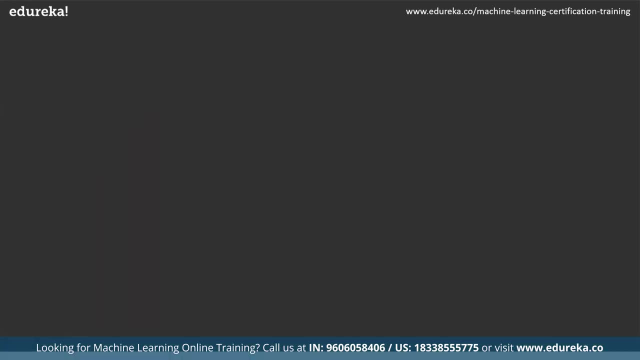 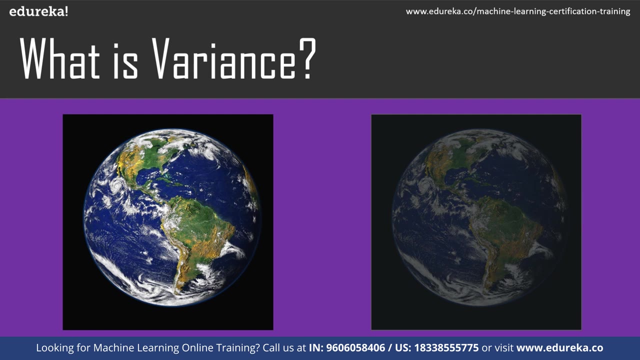 to determine the relationship and thus causing underfitting. Now let's also take a look at variance in machine learning model. So on an independent, unseen data or validation set, when a model does not perform as well as it does with the trained data set, there is a possibility. 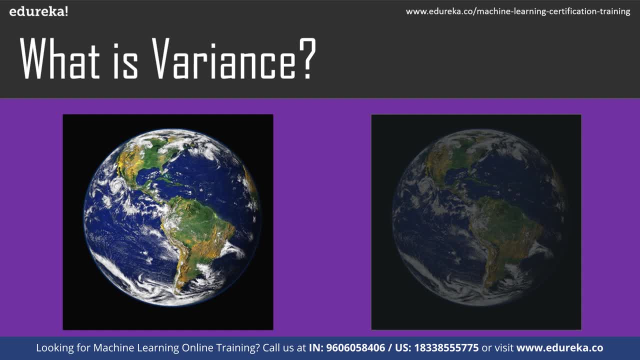 that the model has a variance. It is basically telling you how scattered the predicted values are from the actual values. A high variance in a data set means that the model has trained with a lot of noise and irrelevant data, thus causing the overfitting. 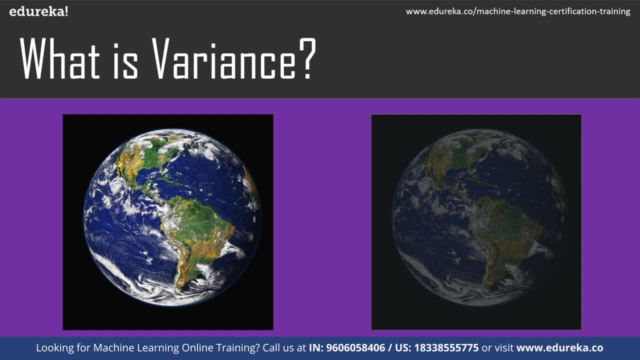 in the model. And when the model has high variance it becomes very flexible and makes wrong predictions for new data points because it has tuned itself to the data points of the training set. So let us also try to understand the concept of bias variance mathematically. 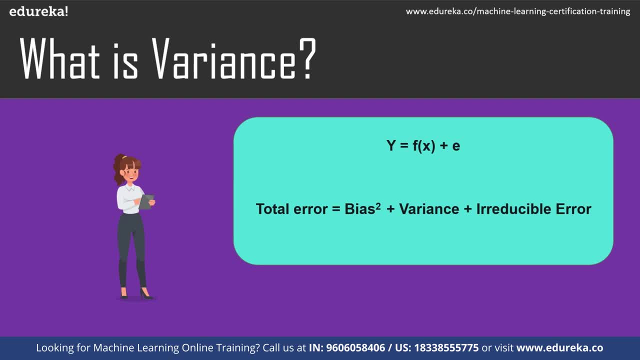 So let the variance that we are predicting to be Y and the other independent variables to be X. So let us assume there is a relationship between the two variables such that Y is equal to FX plus E. So in this equation, E is the estimated error. 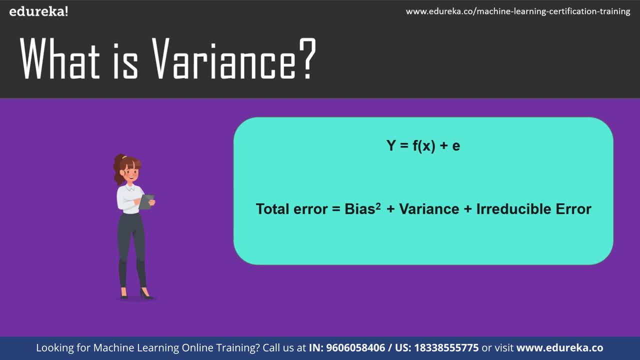 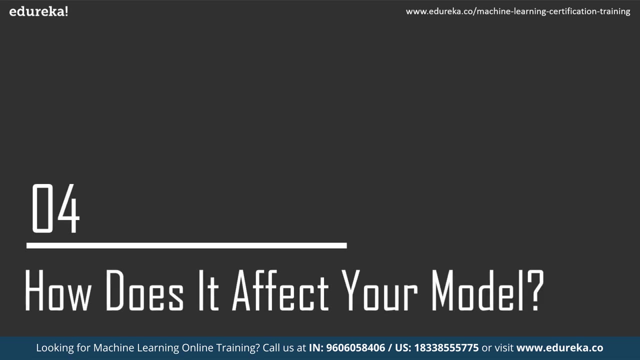 with the mean value zero And when we make a classifier using algorithms like linear regression, support vector machine et cetera, the expected squared error at point X will be bias squared plus variance plus irreducible error. So now let's take a look at how does it actually affect? 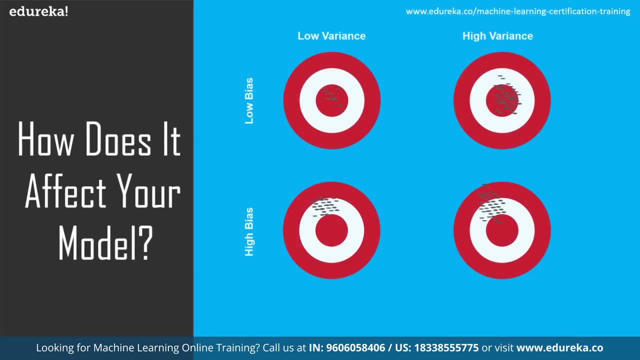 the machine learning model that we are making, So we can put the relationship between bias variance in four categories. that is high variance and high bias, low variance and high bias, Then we have high variance and low bias And, last but not least, 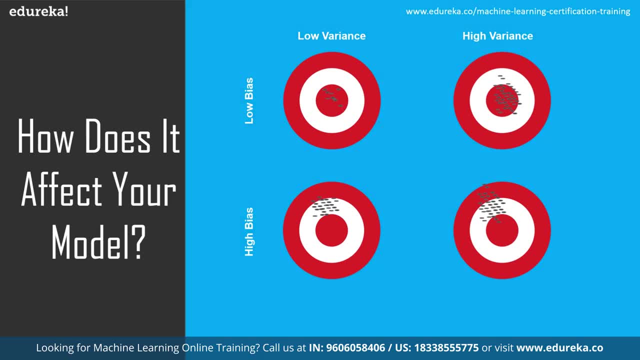 we have low variance and low bias. So the first relationship, that is high variance and high bias. in this relationship, the model will be inconsistent and also inaccurate on average. Now coming on to low variance and high bias, the models are consistent, but they are very low on average. 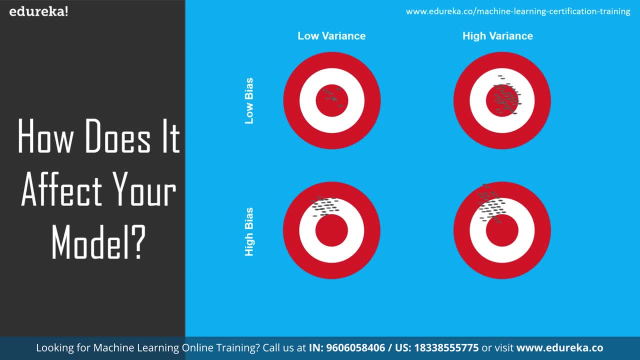 And a high variance and low bias model is somewhat accurate but inconsistent on averages. And, last but not least, that is the low variance and low bias. it is the ideal scenario. The model is consistent and accurate on average as well, So this is where we are targeting our model to be. 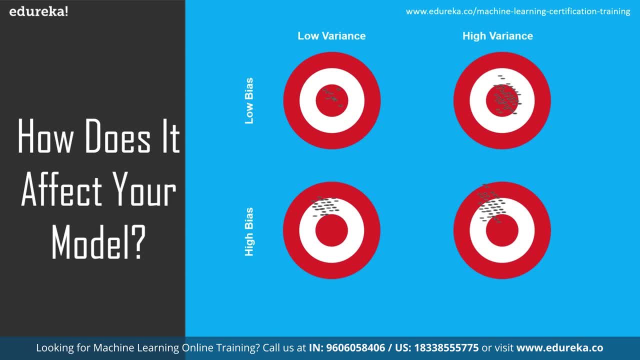 So, although detecting bias and variance in a model is quite evident, a model with high variance will have a low training error and a high validation error, which means that it will not give you as much error when you are testing in on a training set. 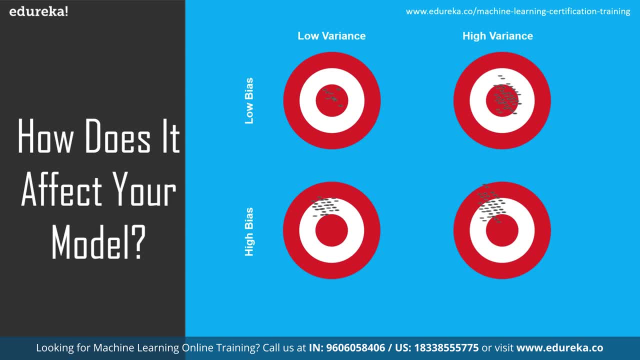 other than on validation set. it will give you a very high error And, in the case of a high bias, the model will have high training error. and validation error is same as the training error. While detecting seems easy, the real task is to reduce it to the minimum. 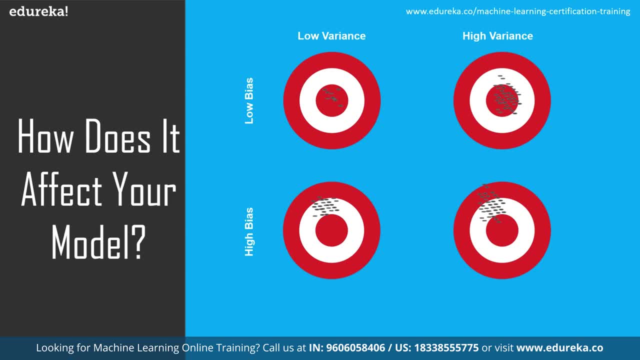 And in that case we can do the following, which is add more input features, we can add more complexity by introducing the polynomial features and we can decrease the regularization term and we can get more training data to reduce bias and variance. And I'll also show you on a linear regression model. 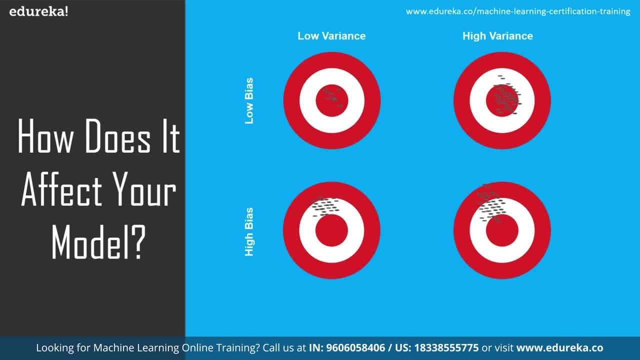 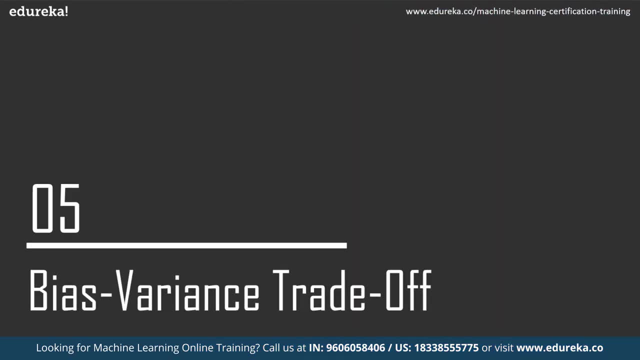 how we can actually reduce the error by adding more training data. So now that we know what bias and variance and how it actually affects our model, let's take a look at bias-variance trade-off, So finding the right balance between the bias and variance. 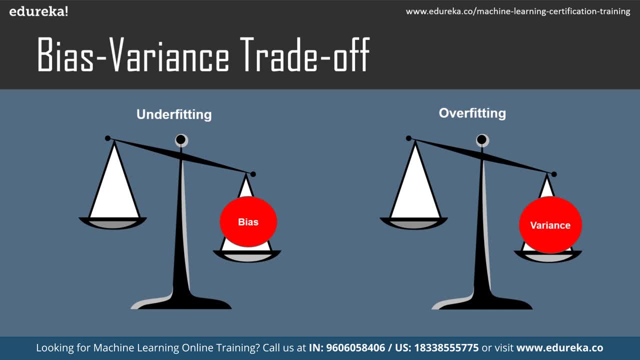 of the model is called the bias-variance trade-off, So it is basically a way to make sure that the model is neither overfitted or underfitted. in any case, And if the model is too simple and has a very few parameters, 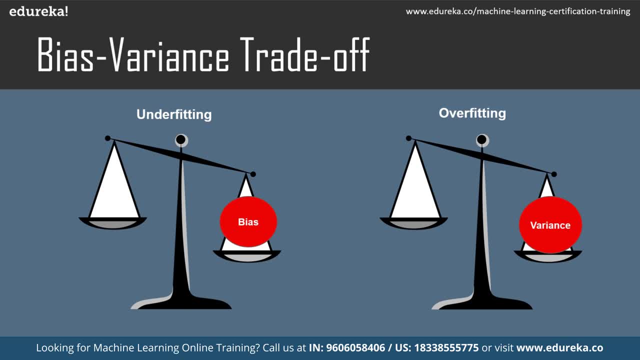 it will suffer from high bias and low variance, And on the other hand, if the model has a large number of parameters, it will have a high variance and low bias. So this trade-off should result in a perfectly balanced relationship between the two. 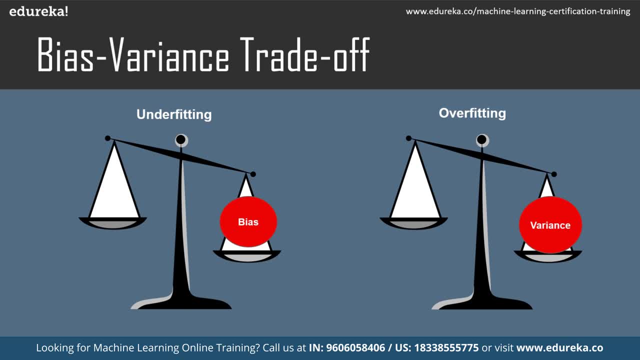 And ideally low bias and low variance is the target for any machine learning model that you have. So in the image over here, if you have a high bias in any model, it's going to underfit the model, And if you have a high variance. 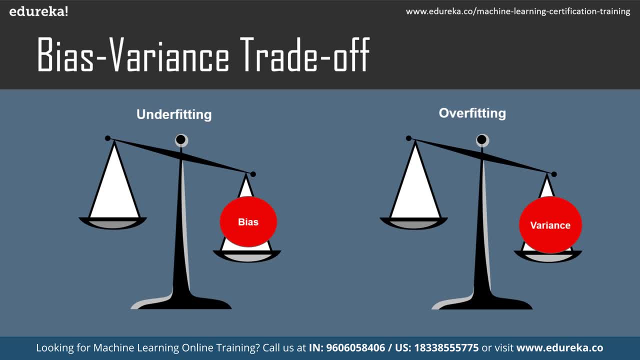 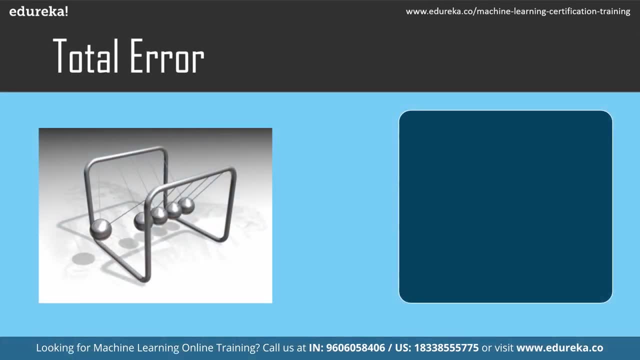 it's going to overfit the model because it will also train with the noisy data. So this is all about bias-variance trade-off guys. Now let's talk about total error. So in any machine learning model, a good balance between bias and variance. 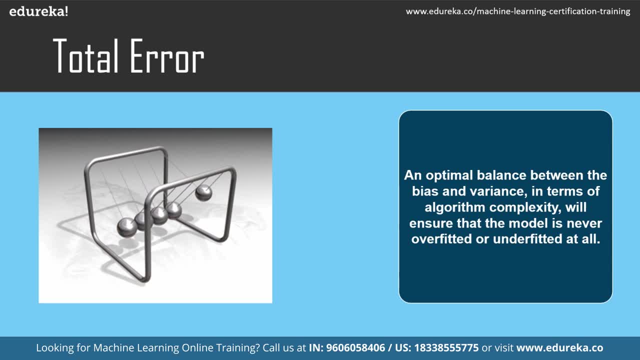 serves as a perfect scenario in terms of predictive accuracy and avoiding overfitting, underfitting altogether. An optimal balance between the bias and the variance in terms of algorithm complexity will ensure that the model is never overfitted or underfitted at all. 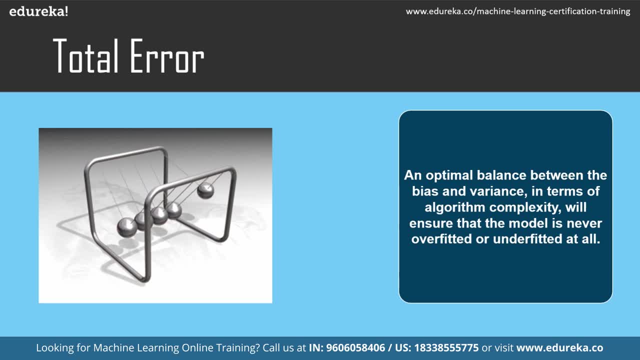 So let's understand how we can reduce the total error with the help of a practical implementation. So I've already created a linear regression classifier, so I'll begin with the starting. You can also find it on the linear regression in machine learning article on Eddie Rigger using the diabetes dataset. 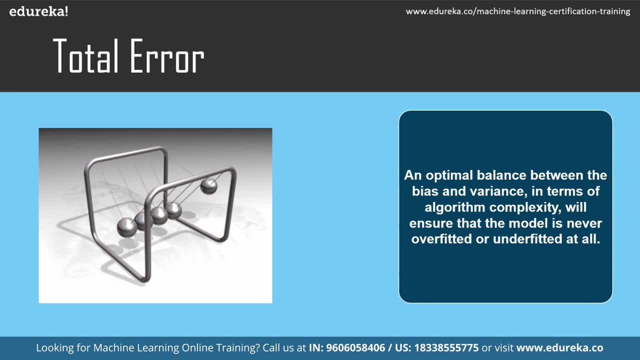 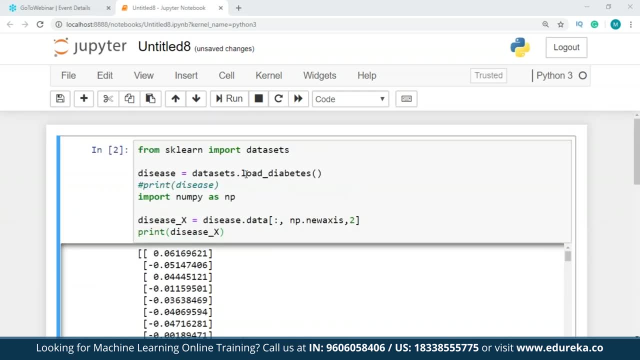 in the dataset module of scikit-learn library. So let's go to Jupyter Notebook guys. So we're in the Jupyter Notebook. I've already written down the code for the model over here. So it is easy. We are using the load diabetes model. 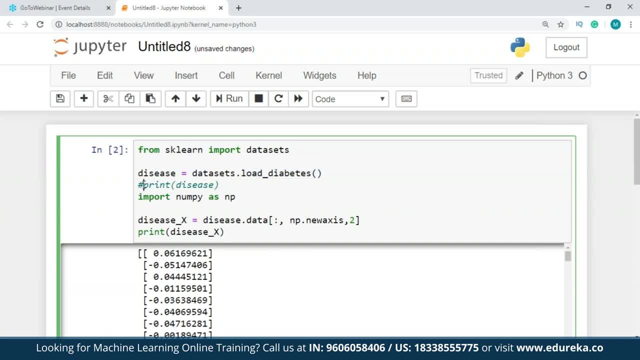 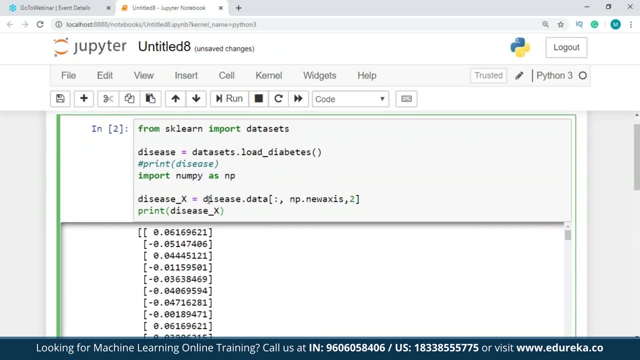 that we have in the dataset module. So first of all, you know, I've come to down this line which prints the dataset, and then I have imported the numpy array And after that we have used only one column from the dataset for training.